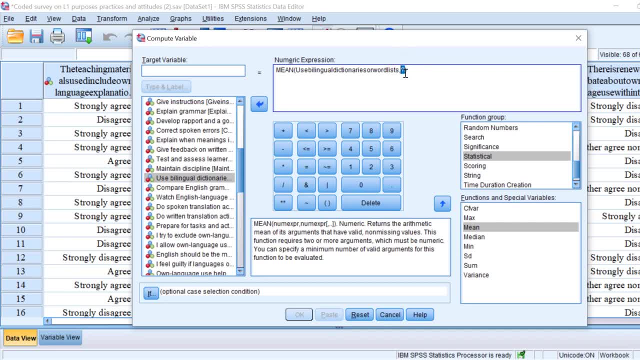 move or have a comma besides or after each item separately. So one finger is on the comma and the other finger, or the mouse, is on the other items. So let's double click each item, put the comma till we finish the scale, Then prepare task for or tasks before. 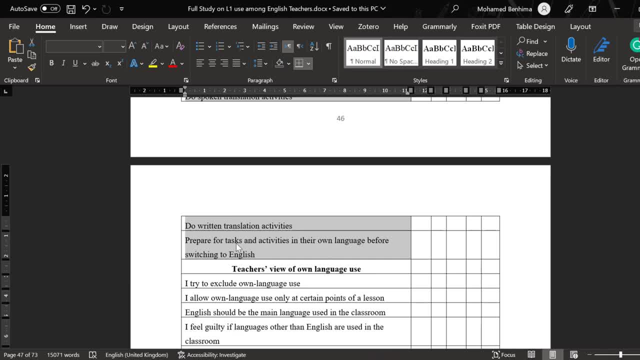 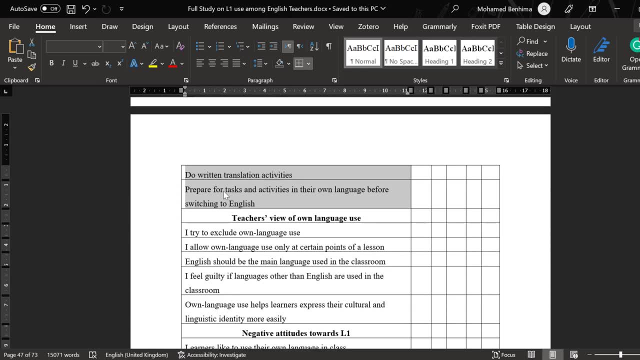 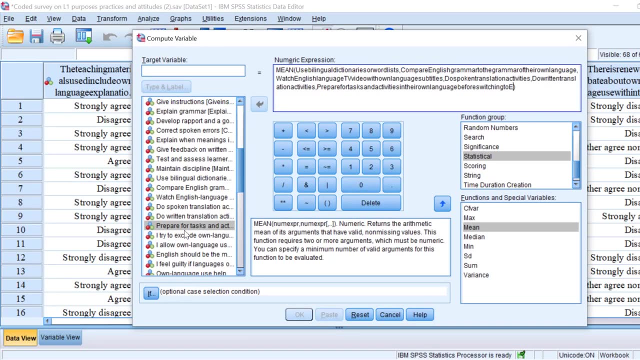 switching to English. So I think these are the items, so the use of bilingual dictionaries and the preparation for tasks, because this is an adapted scale so there may be some differences, And then here we are going to choose or find the name for this. So it is called the whole dimension, is called reported frequencies. 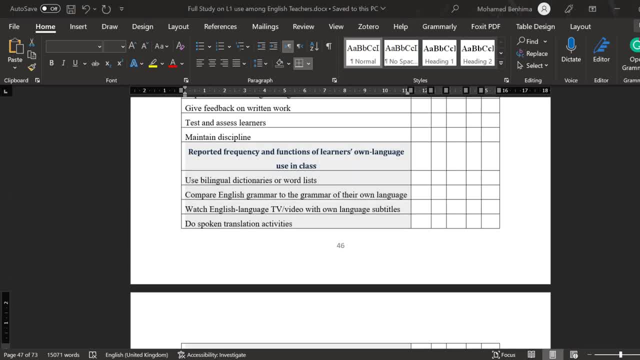 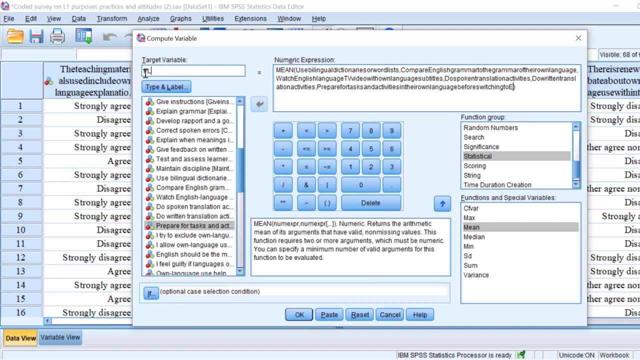 And functions of learners on language use in class. So we're going to include functions- language in class. That's it. So we can even type a label here, because this variable or this column or this cell does not require or does not allow spaces, So I can choose label here. So let's ignore this, for 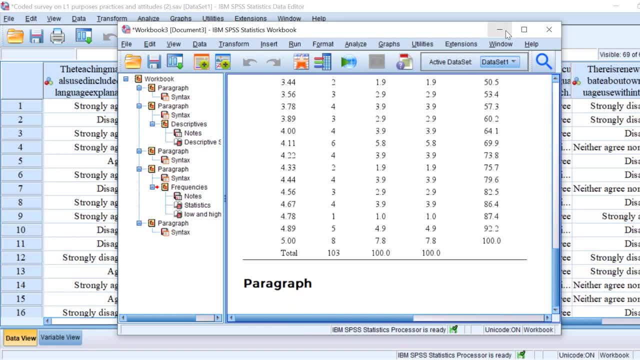 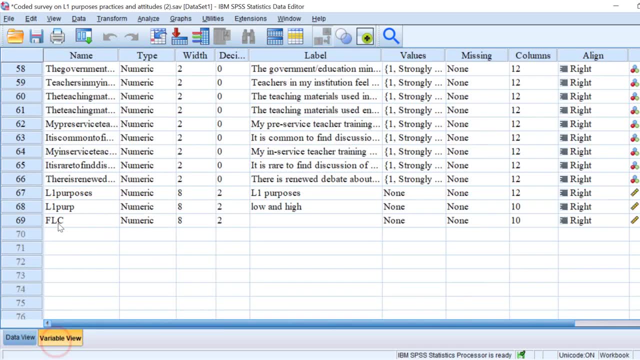 the time being and click OK And let's wait for the outputs. It's not going to be an output in the output window, But what will happen is that if we go to the variable view, we will find the variable that has been created at the end of the questionnaire. 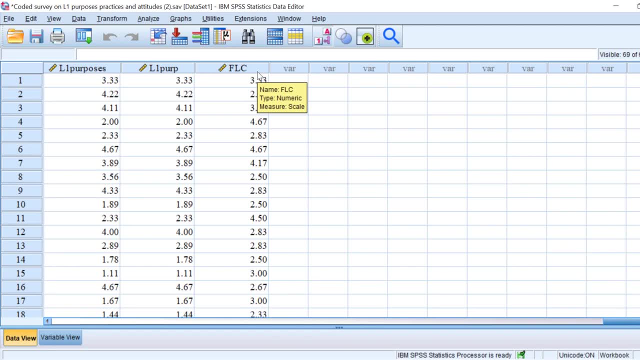 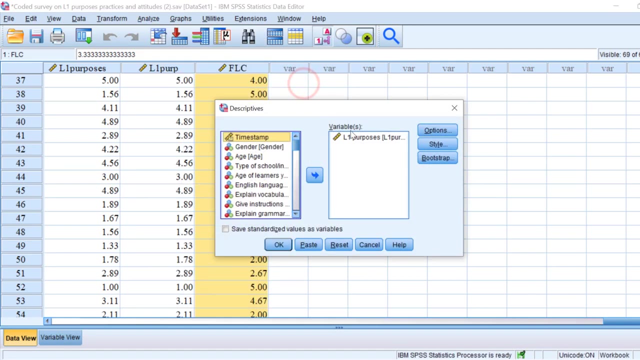 So if we double click on it, we're going to find the, the mean score of all items, And we can even compute the mean score of the whole construct by going to analyze descriptive stats, descriptives, and I'm going just to move the newly created 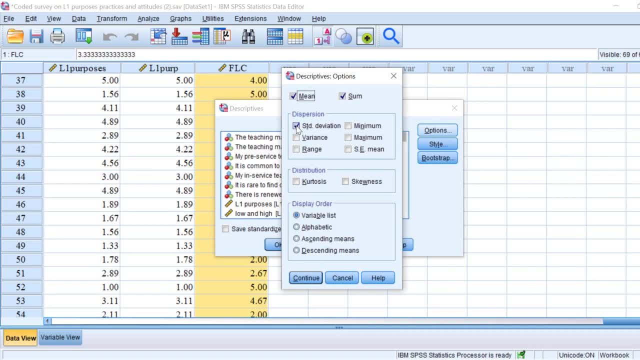 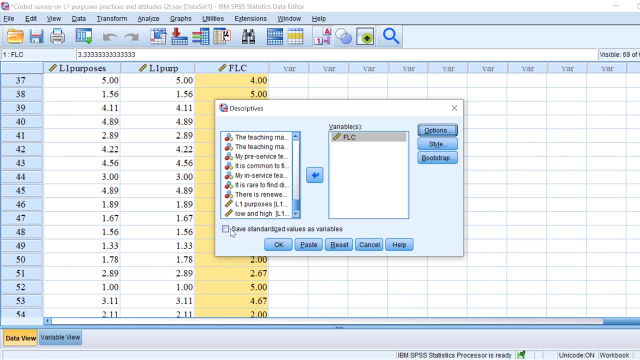 variable, and from options I can choose the mean, standard deviation and the sum, and this will compute the overall mean score. I can even transform this mean into the z-score, in the sense that I need to save standardized values as variables, so so that a new variable will be created that is going to be called. 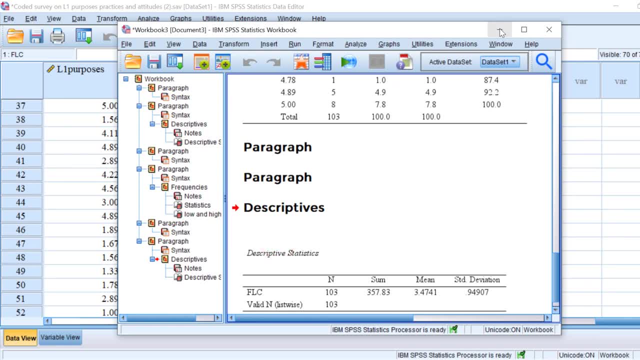 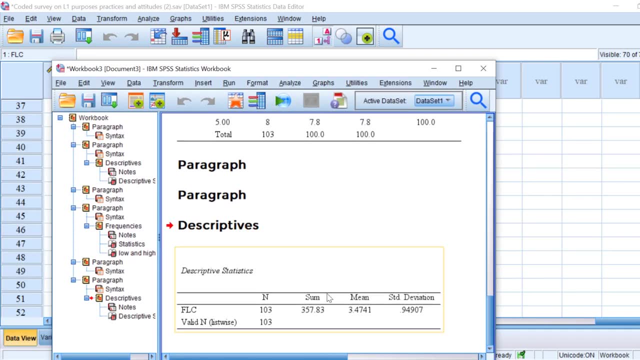 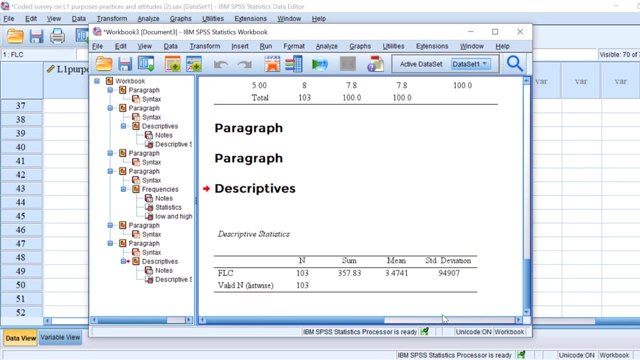 the z-score, click OK and let's have two functions at once. so here is the z-score and here is the mean, or the overall mean score of this variables: 3.47. this means that most respondents agree with most items. you or even express neutrality. okay, this is the standard deviation that shows how. 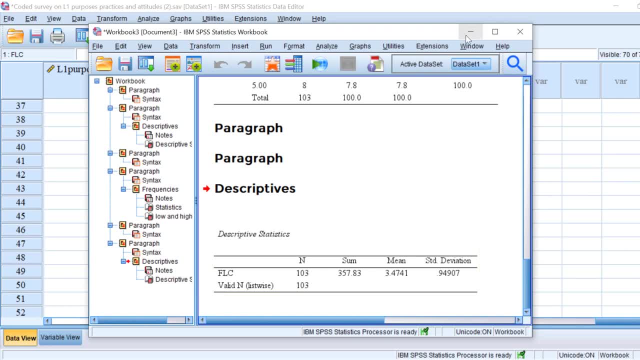 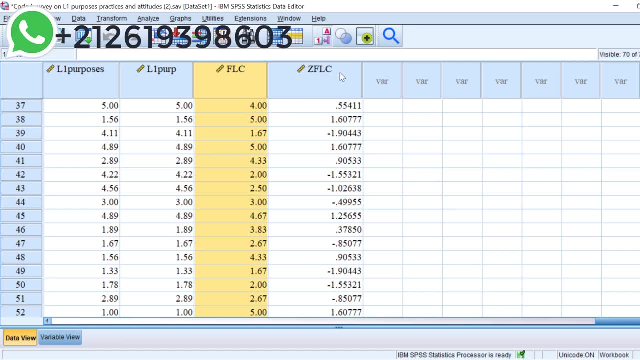 each respondent differs from the other. so this is, in brief, how we can group placard scale items in one construct and even compute the z-score and interpret the results by running descriptive stats. till then, see you in another video. if you have questions or remarks, do not hesitate to post them below or contact me via one of my social 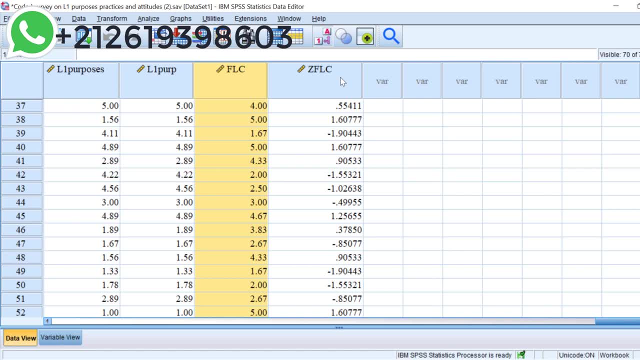 media. I answer as many questions as I can and see you soon. bye for now, you. 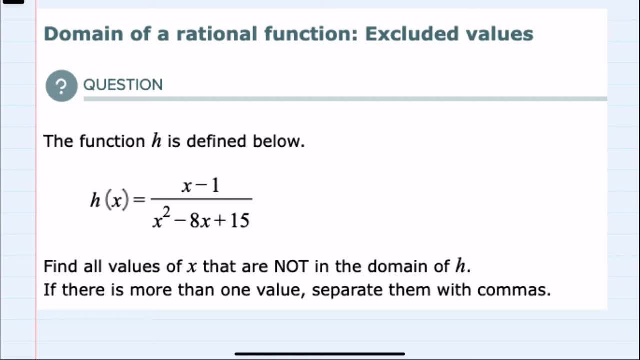 In this video I'll be helping you with the Alex problem type called domain of a rational function excluded values. We're given the function h of x and asked to find all the values of x that are not in the domain of h. And the limiting factor here is that we have a fraction and we know that. 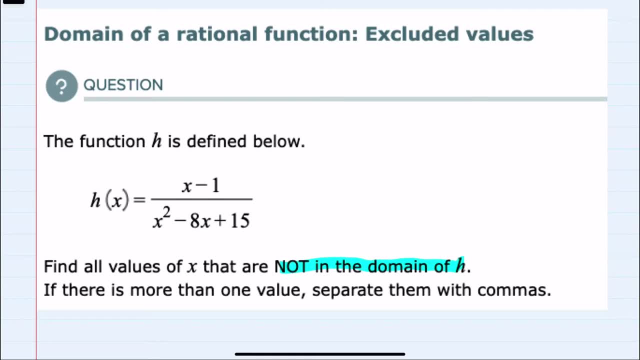 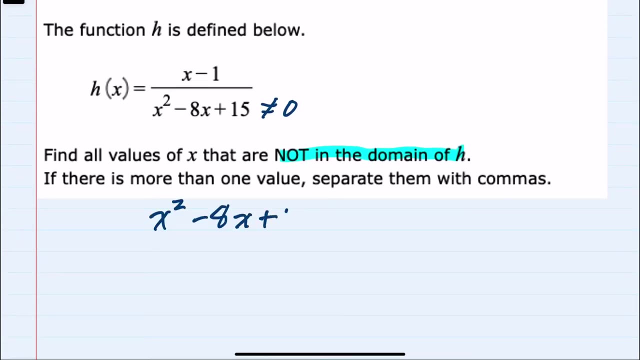 the denominator can't be zero. So our x squared minus 8x plus 15 cannot be equal to zero. So to find the values to exclude, I'm going to take that x squared minus 8x plus 15.. I'm going to set that. 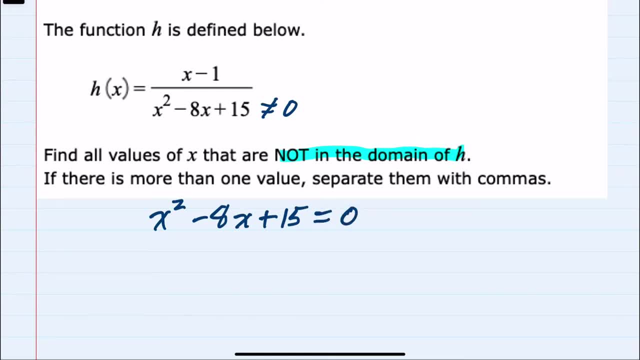 equal to zero. to find which values I would need to exclude from the domain And to solve this. since the leading coefficient is 1, this will factor nicely The left hand side. the x squared would have to be x and x. The factors of 15 are either 1 and 15 or